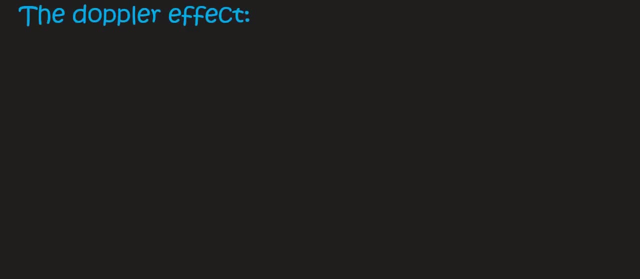 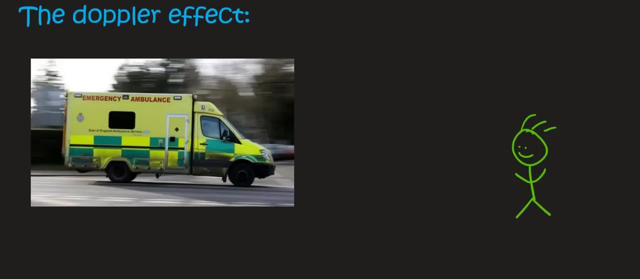 Hello everyone. in this lesson we are going to be talking about the Doppler effect. So if you've ever been standing on a road and an ambulance comes towards you, what you would notice is that it appears that the sound of the ambulance, or the siren, is getting louder the closer it gets to you. Do you really think that the driver sitting over here is he's not like a DJ? he's not changing the volume. What's happening is that the siren is the same sound, but what's happening is that that sound travels as waves. Now, as 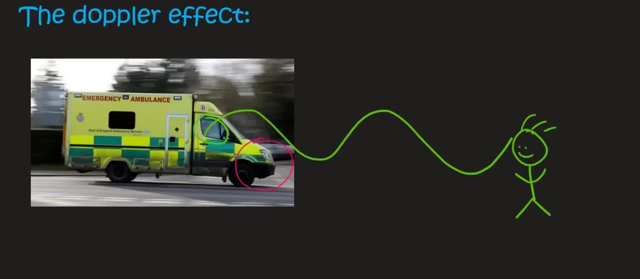 that ambulance gets closer to you, the ambulance itself is colliding with those waves and it's causing those waves to be more compressed, And so if the waves are being more compressed, it means that more of the waves are hitting your ear per second. So when it's very far away, the waves are very relaxed and you may be hitting- you may be getting three or four waves per second. As the ambulance gets closer, those waves become compressed and so maybe your ear is now hitting, or hearing 20 waves per second, And so the frequency. listen to the word carefully, frequency. Frequency means how often, And so the number of waves that are hitting your ear per second increases, and that's what makes it seem like the volume is increasing, But in actual fact it's the frequency. So that is the Doppler effect. It's the apparent change in the frequency when a source and a listener move. 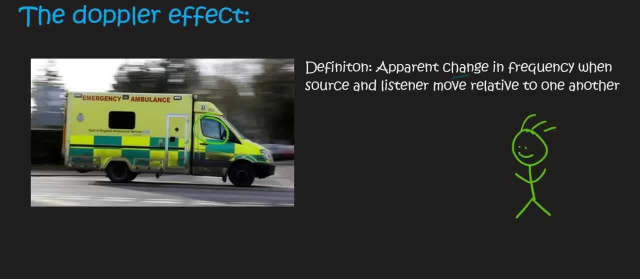 relative to one another. Let's go through that carefully. It's the change in the frequency when a source, a source is where the sound is coming from, So that would be the ambulance in this case, And the listener, which is this person, move relative to one another. Why do they have to move? Well, let's imagine that this ambulance is not moving Then, and let's imagine that the person is also not moving. Then the amount of waves that are hitting that person's ear per second will stay the same, And so 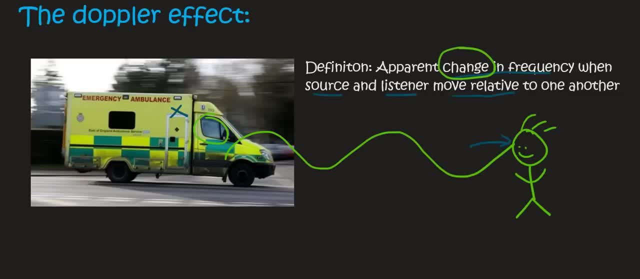 the frequency will not change. However, as this person starts moving closer to the ambulance- let's say, the ambulance is not moving, but the person starts moving closer- Well, that person is going to start causing the waves to compress slightly, And so it's going to look more like that, And so the frequency will be higher. Of course, the ambulance could move as well, And that would do the same, Or both objects could move, and that would cause even higher change in the frequency. So there has to be movement, Either